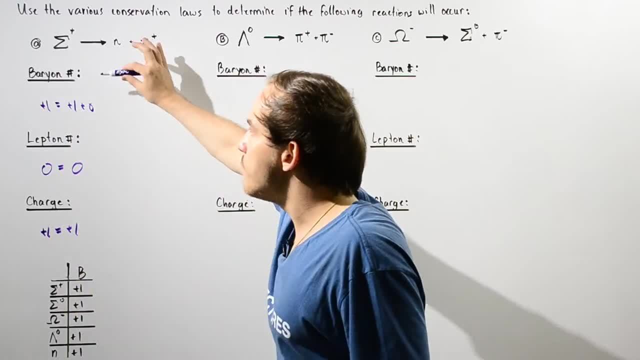 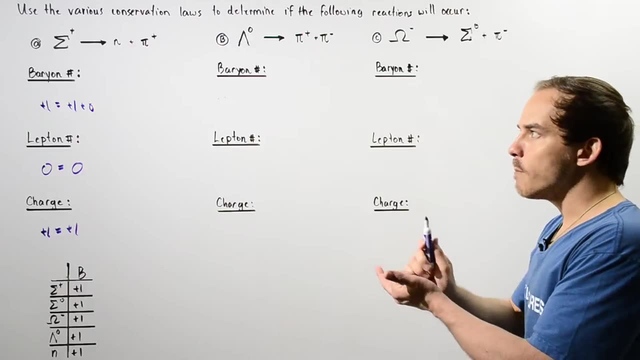 which is equal to positive one, and so the barium number, the lepton number and the charge are all conserved, and assuming that the energy and momentum are also conserved, then this reaction will take place. What about the lepton number? Well notice, none of these particles are lepton. 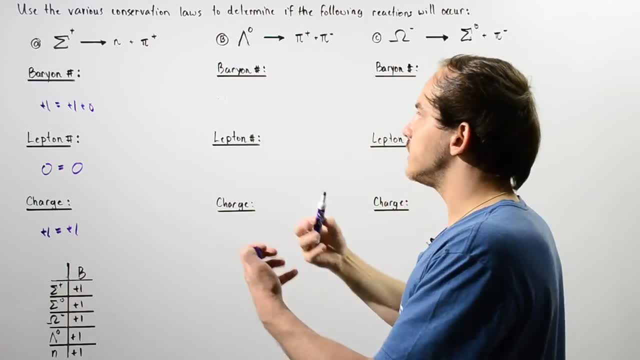 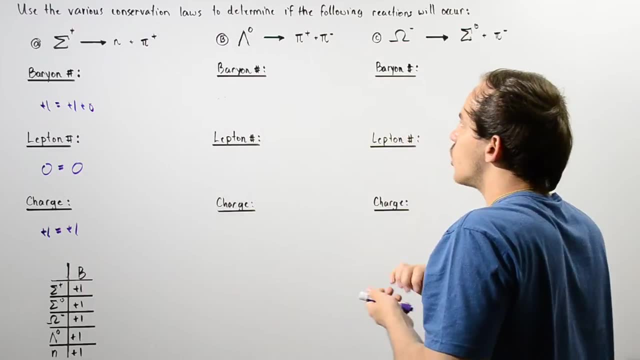 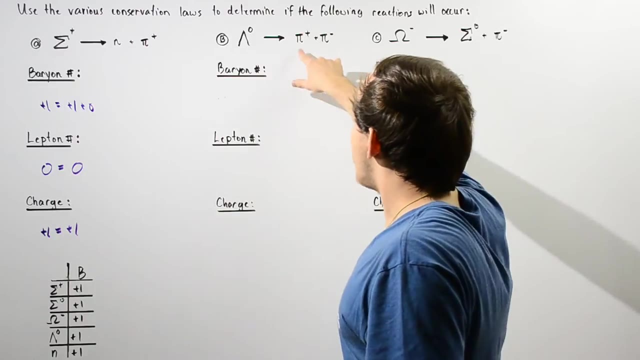 What about part B? Well, now we have a slightly different reaction. We now have a lambda that decays into these two pions. So we have a pion with a positive and a pion with a negative. So the pion positive and the pion negative are basically not baryons. 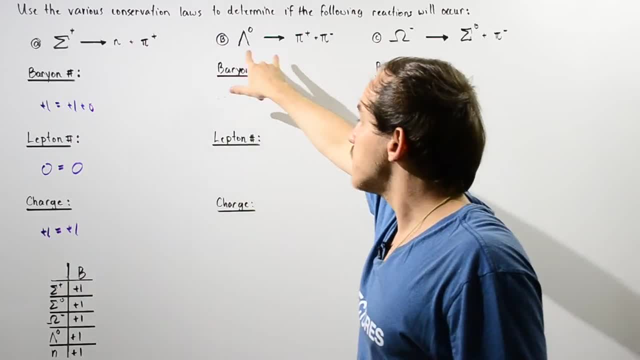 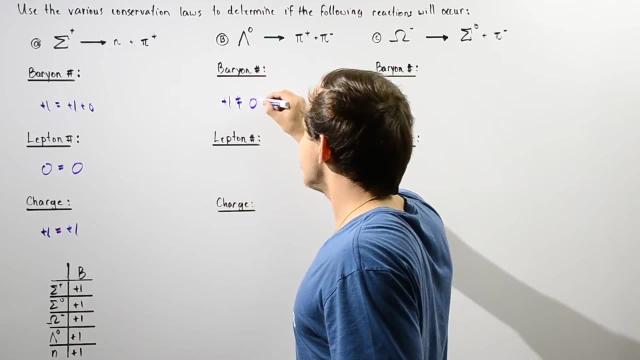 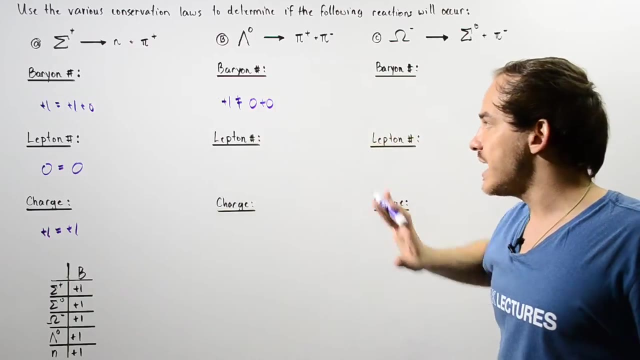 So they both get a baryon number of zero. However, the lambda gets a positive one And we see that positive one is not equal to zero plus zero and that means the baryon number is not conserved and this reaction will not take place. 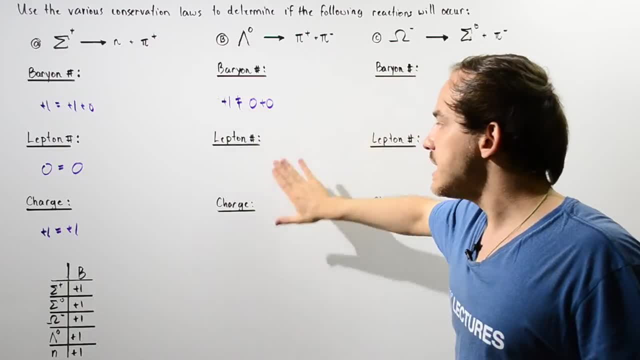 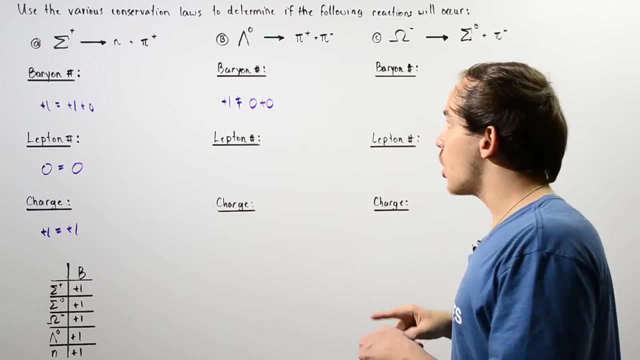 But let's finish the lepton and charge and see if these are conserved. Well, the lepton number? well, none of these are leptons, once again. and so we see that zero does equal to zero And the lepton number is conserved. 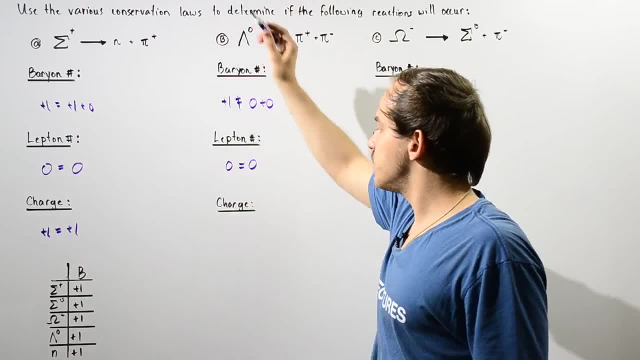 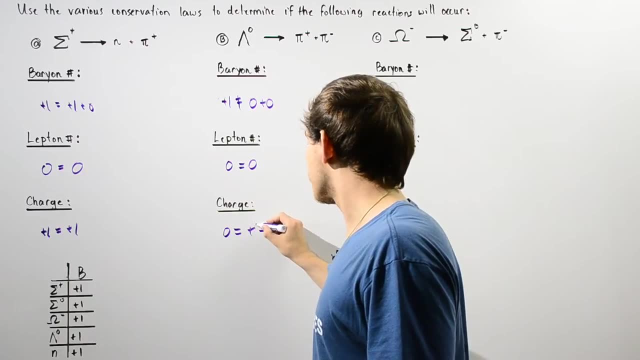 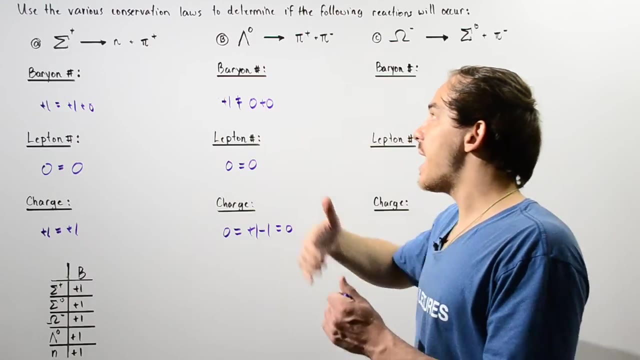 What about the charge? We have a zero charge on this side and a positive one minus one and a zero on the right side, because positive one minus one gives a zero. and so we see, the charge does in fact conserve, But because the baryon number isn't conserved, reaction B will not take place. 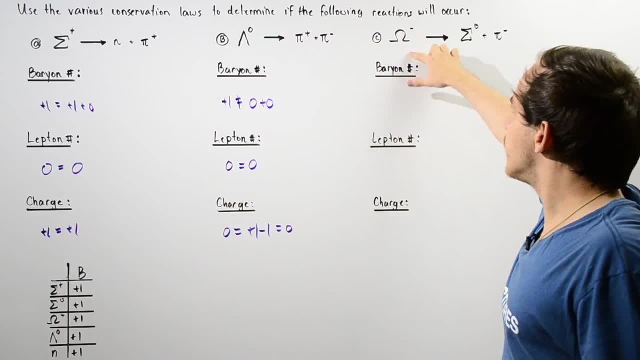 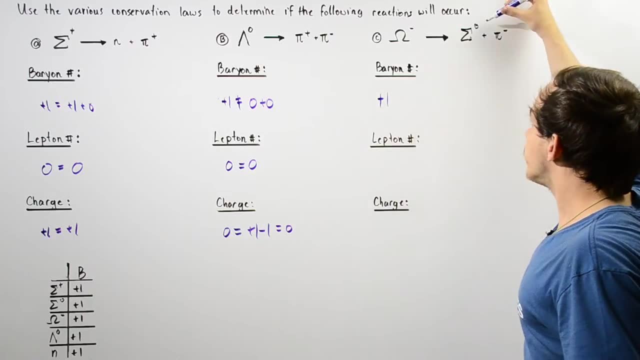 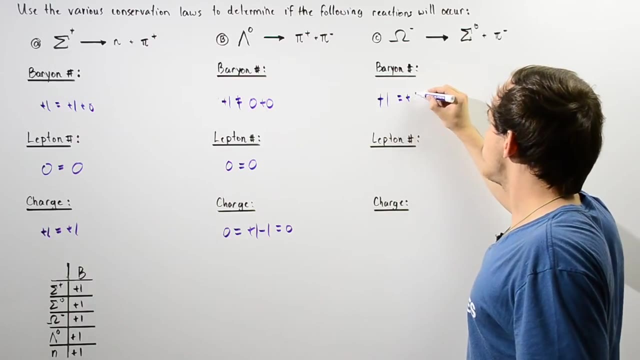 Now, what about C? Well, we have omega, So this gets a positive one for the baryon number. We have a positive one here. What about on this side? Well, we have this, which also gets a positive one, but this is not a baryon, so that will. 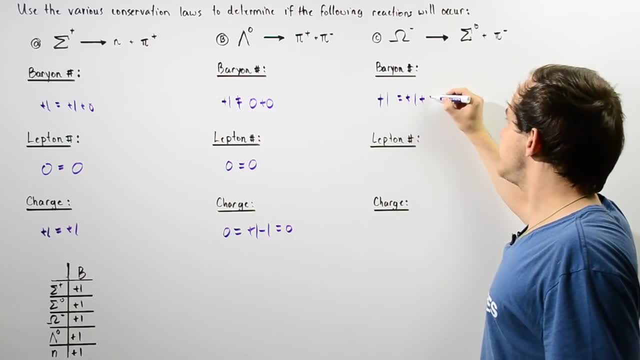 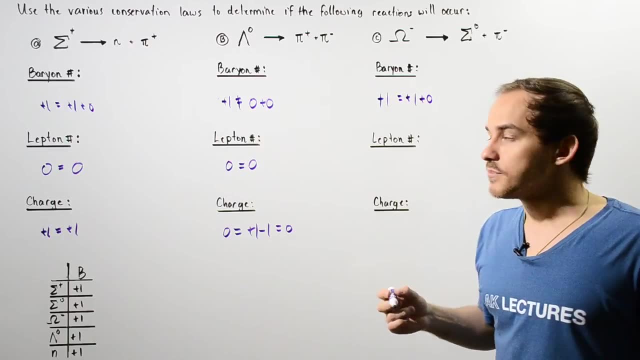 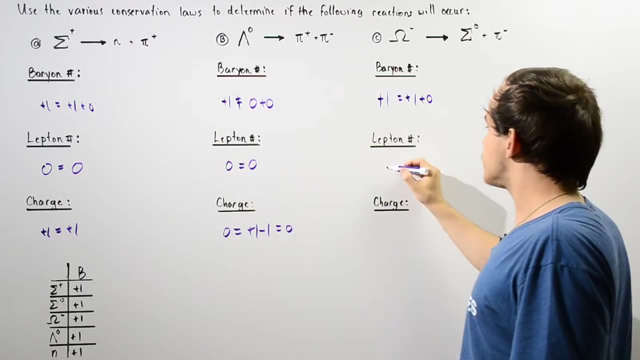 get a zero and we see plus one. plus zero gives us a plus one and the baryon number is conserved. What about the lepton number? Well, this isn't a lepton, This isn't a lepton, And this isn't a lepton as well.